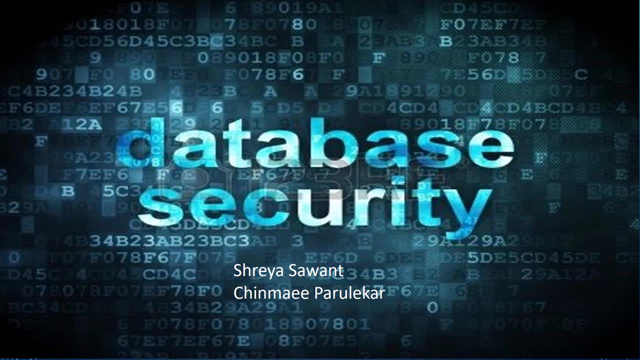 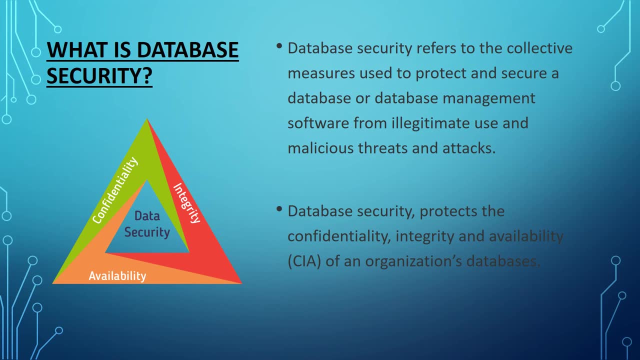 Good afternoon everyone. Our topic of today's presentation is database security. What is database security? Database security refers to the collective measures used to protect and secure a database or database management software from illegitimate use and malicious threats and attacks. Database security protects the confidentiality, integrity and availability of an organization's databases. 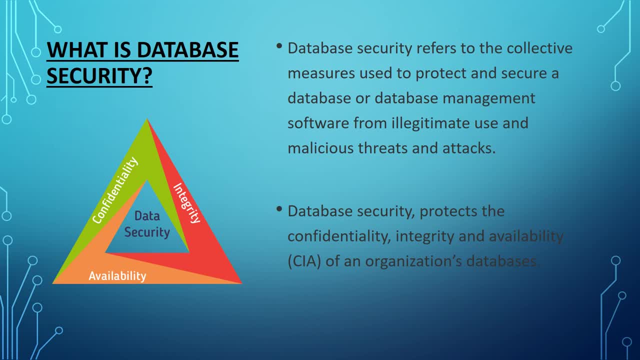 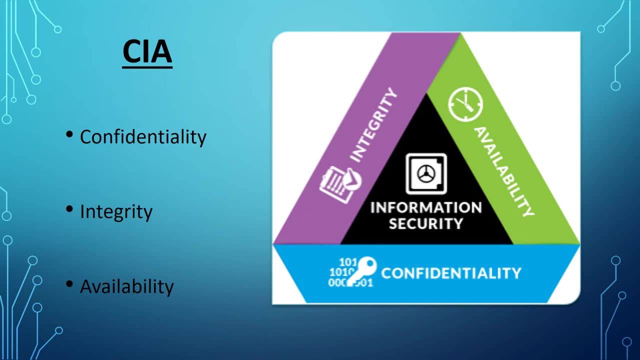 This CIA triangle constitutes a very important aspect of database security. CIA First is confidentiality. Confidentiality refers to keeping the data secretive so that only authors can access it. Confidentiality refers to keeping the data secretive so that only authors can access it. Confidentiality refers to keeping the data secretive so that only authors can access it. 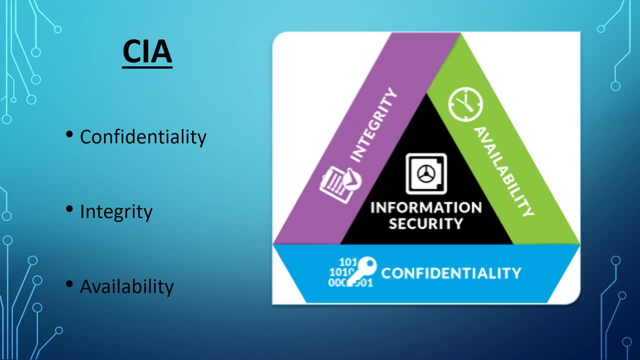 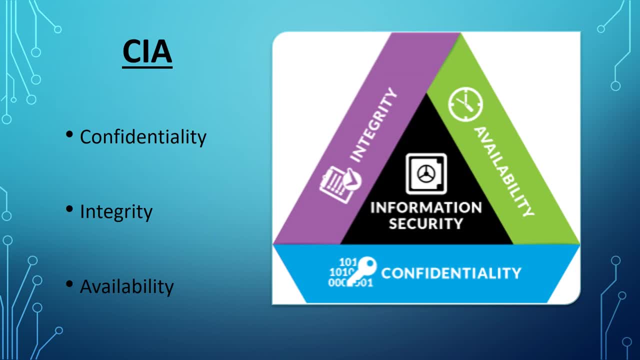 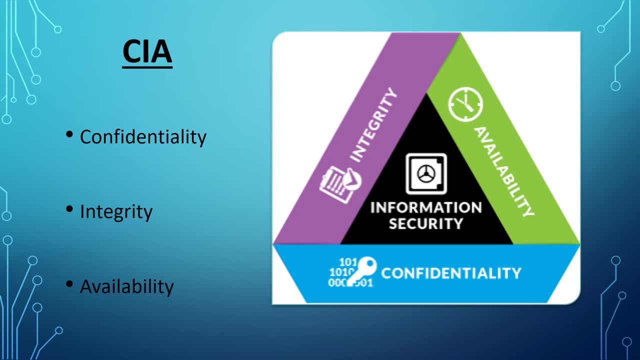 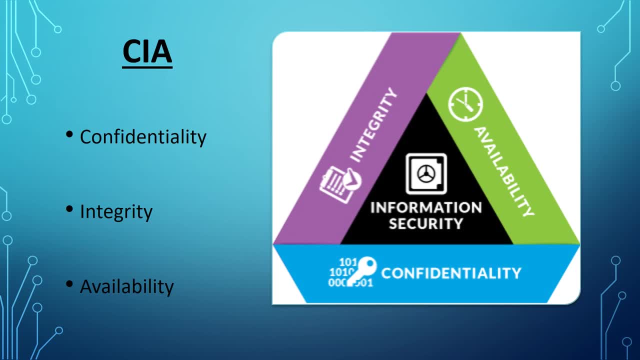 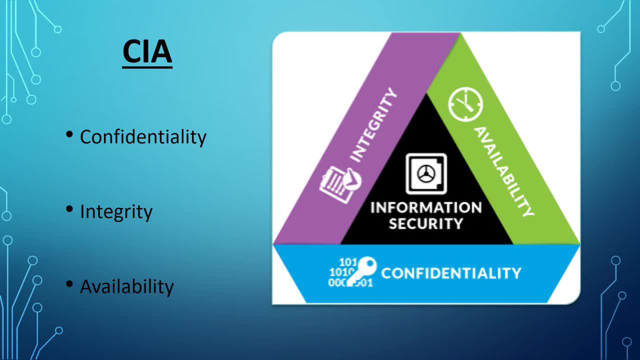 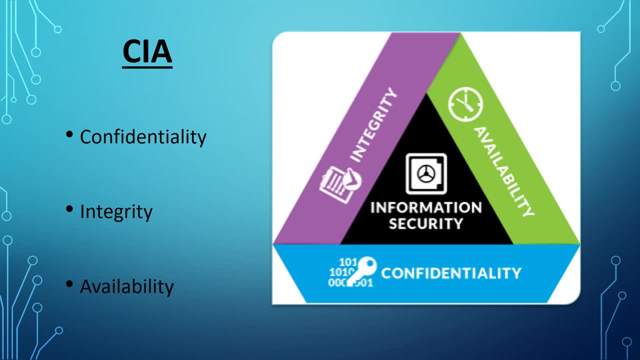 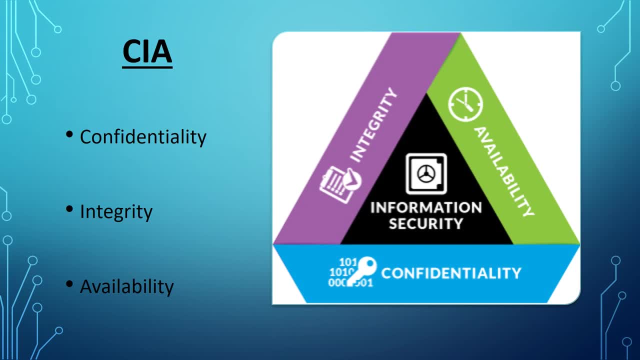 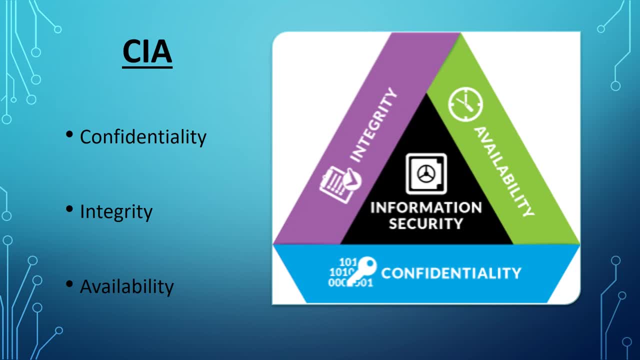 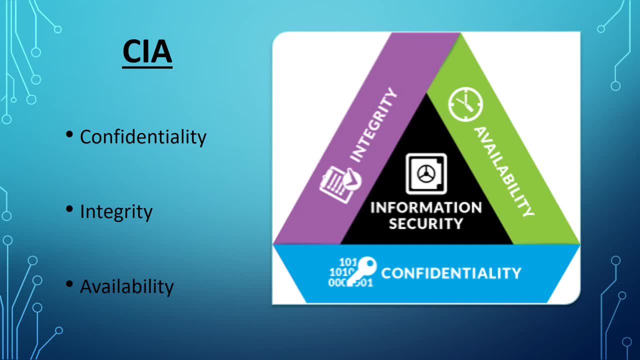 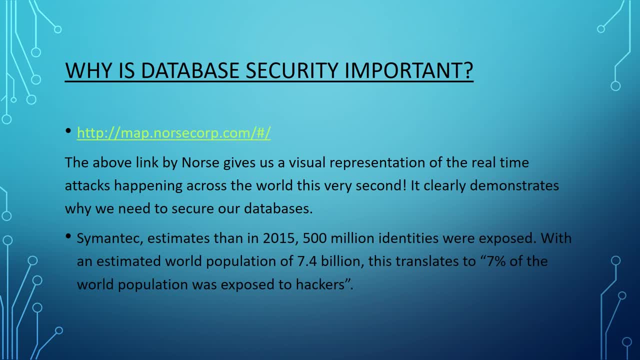 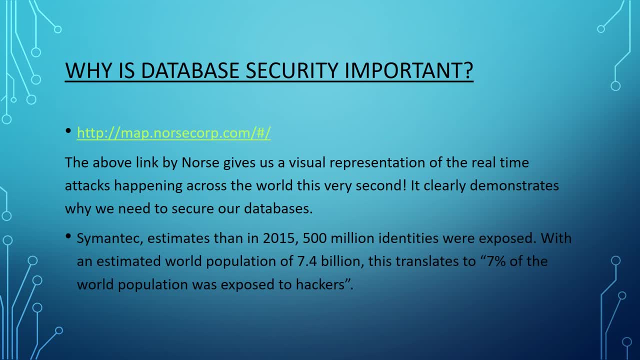 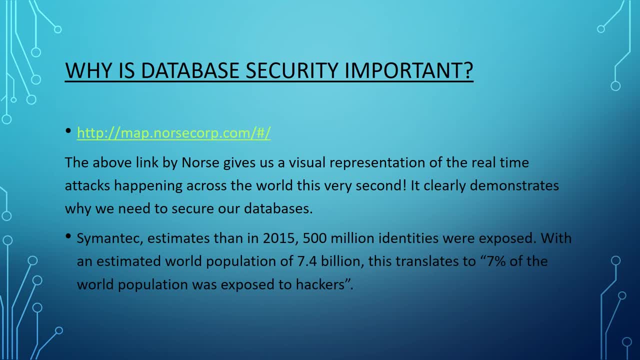 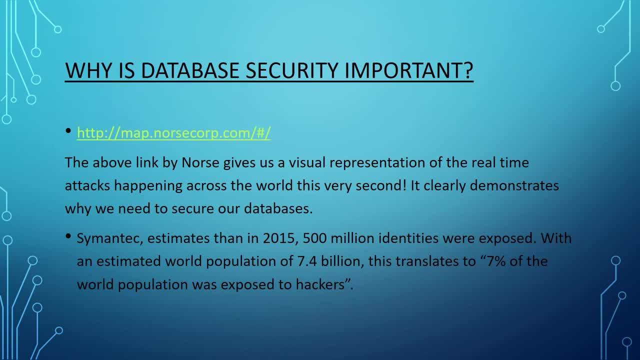 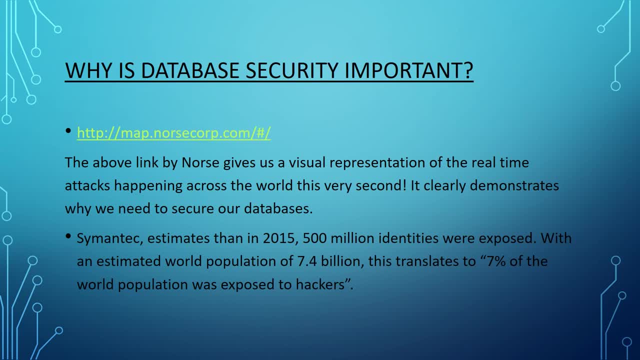 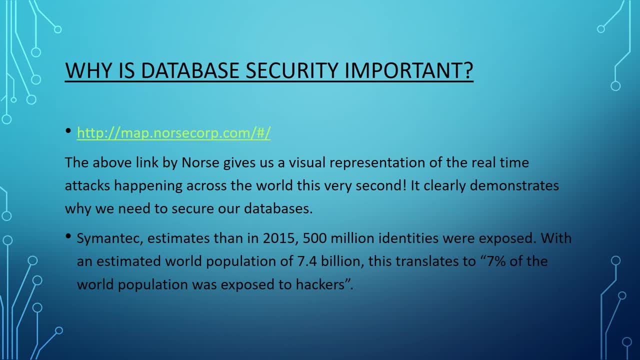 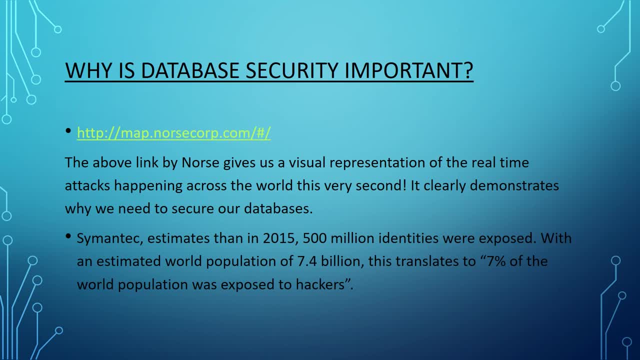 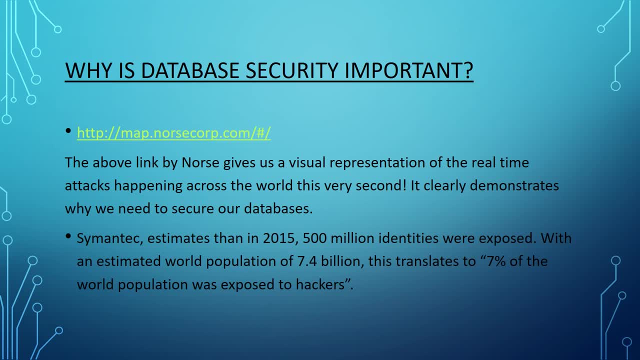 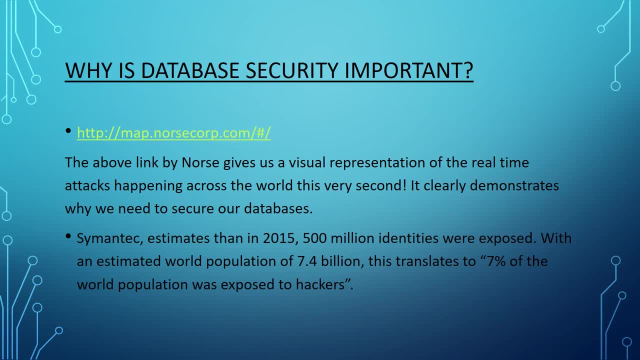 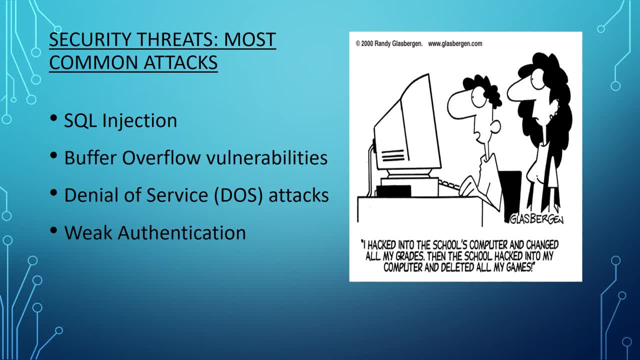 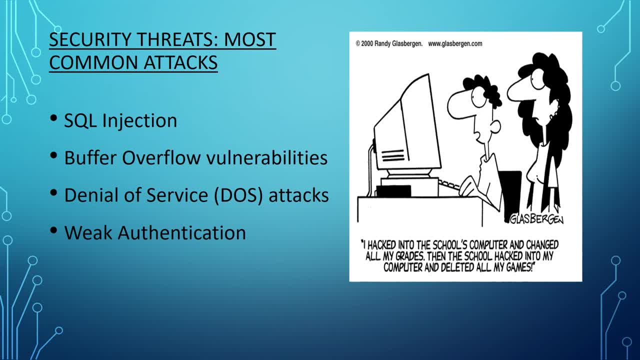 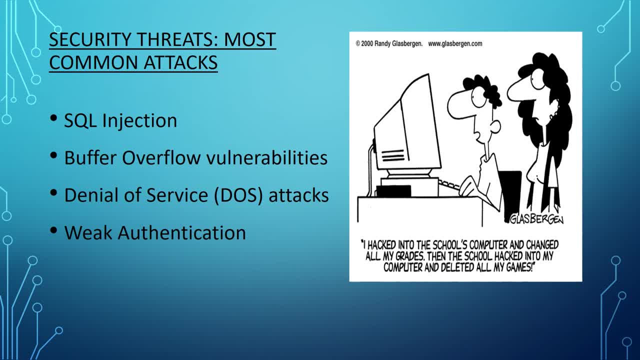 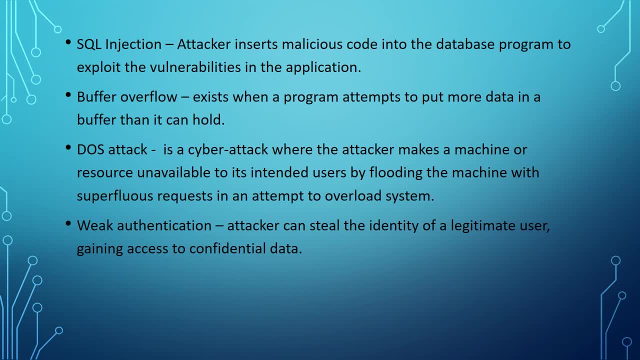 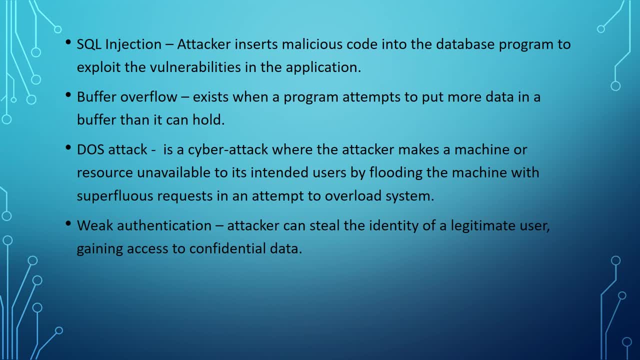 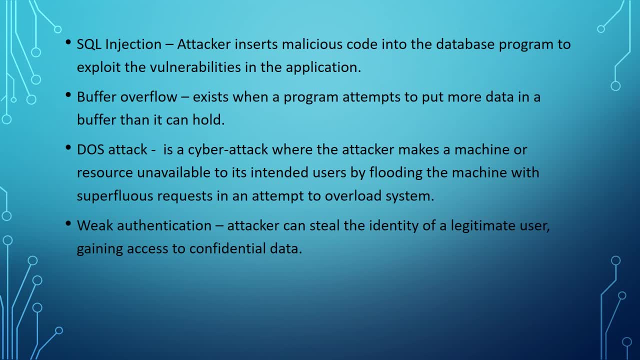 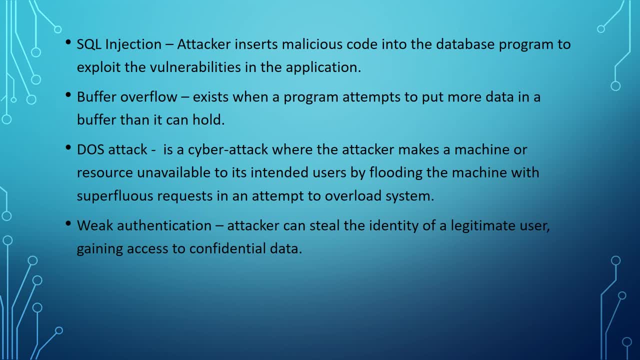 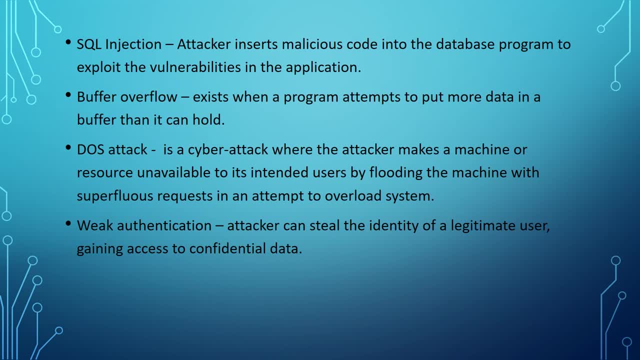 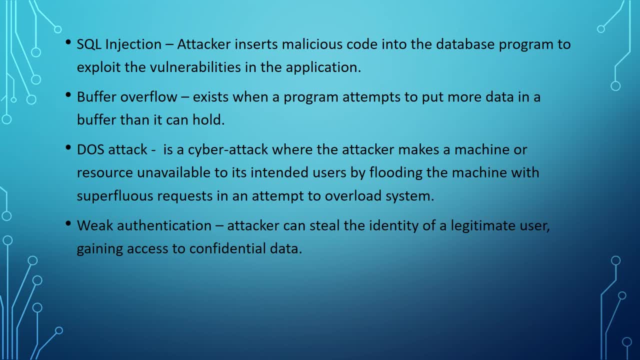 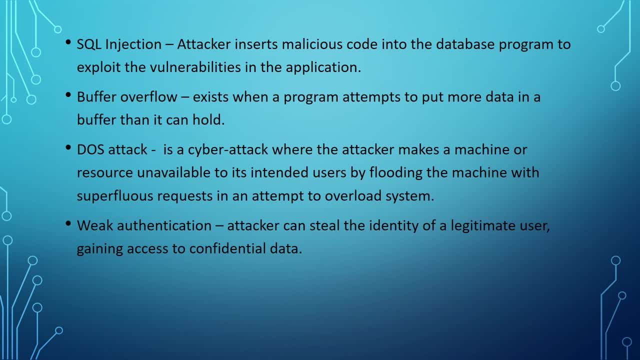 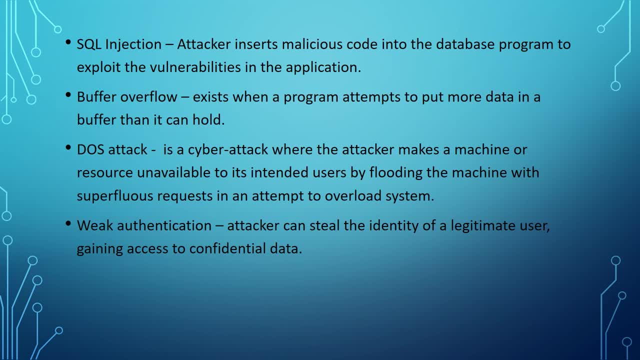 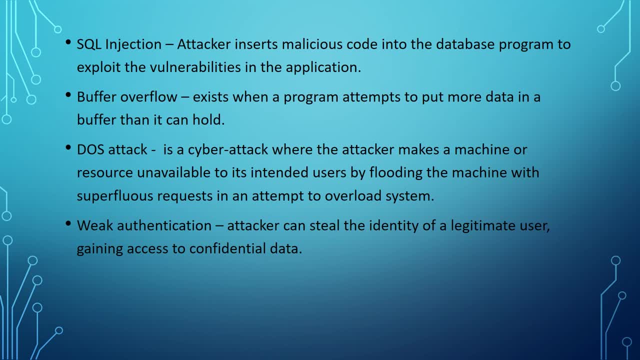 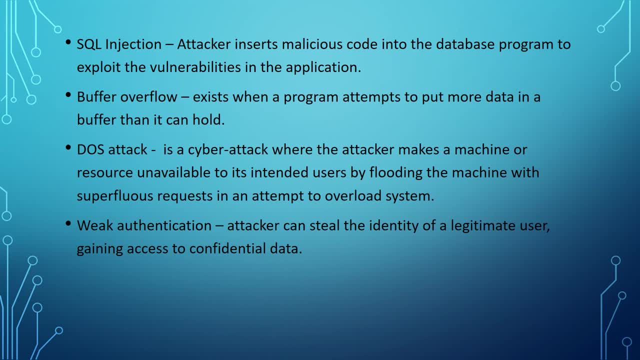 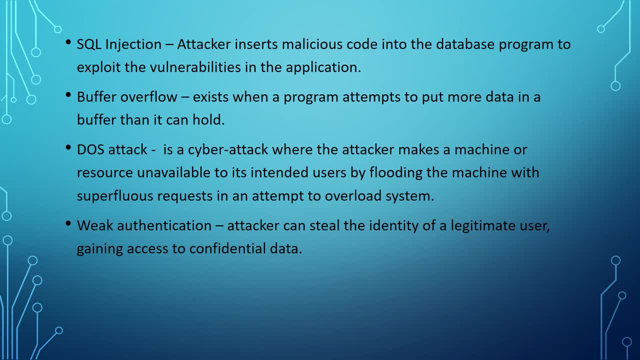 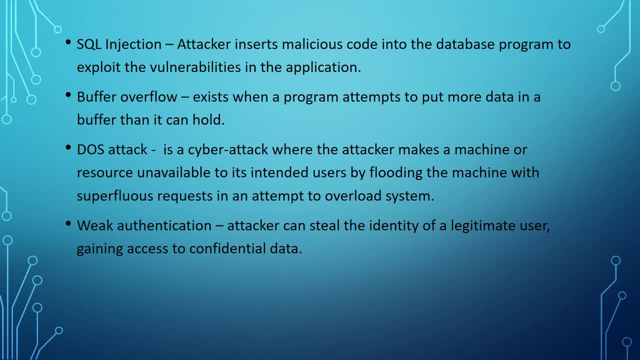 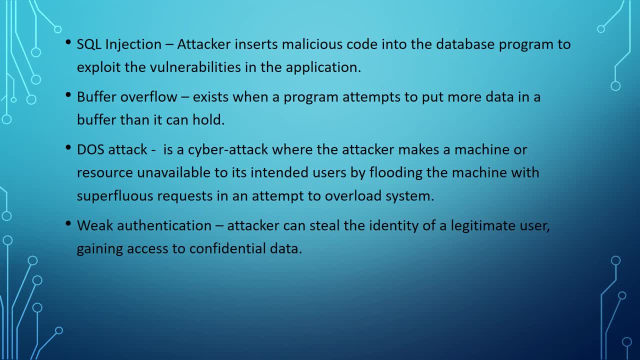 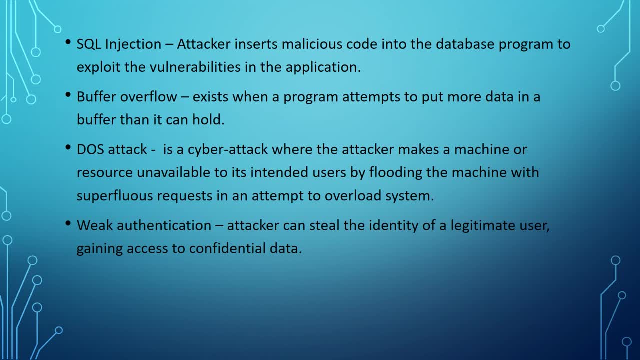 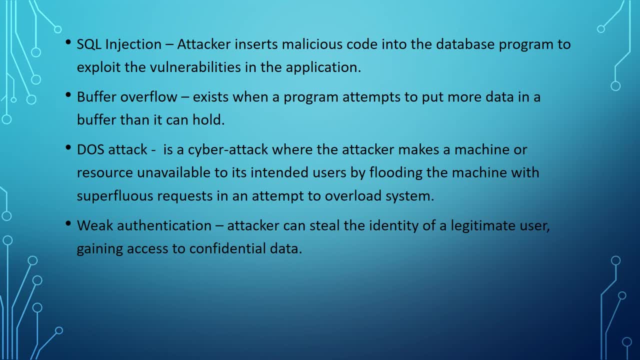 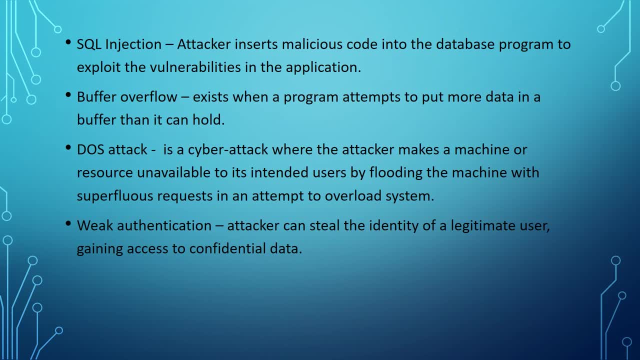 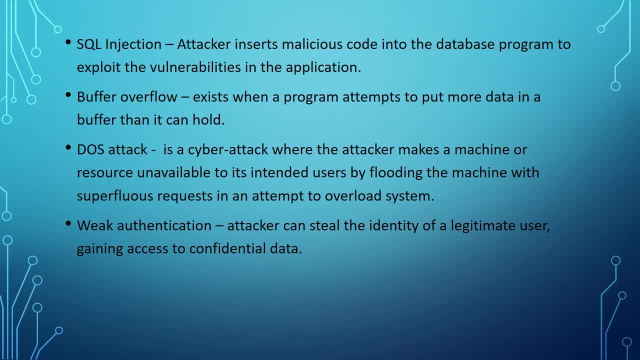 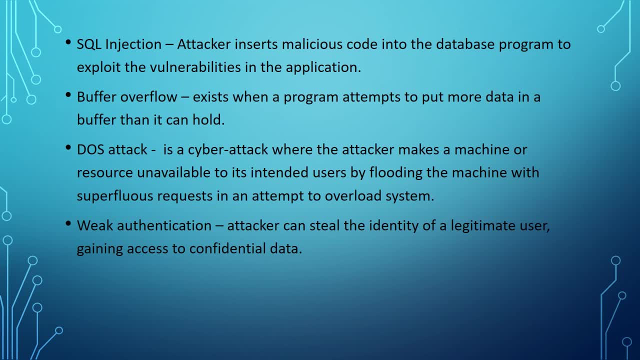 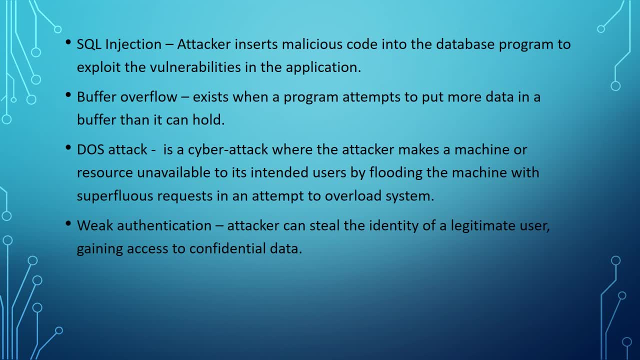 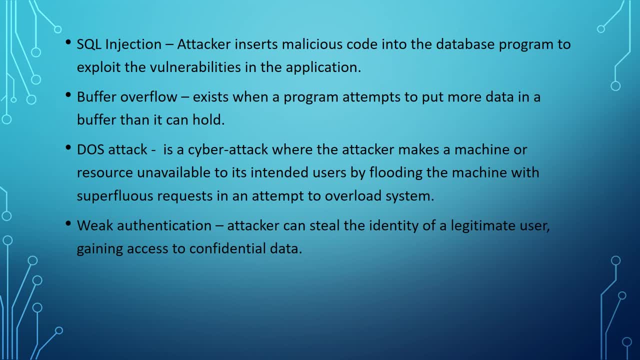 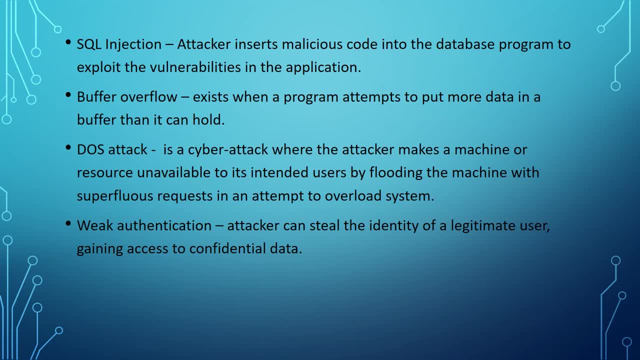 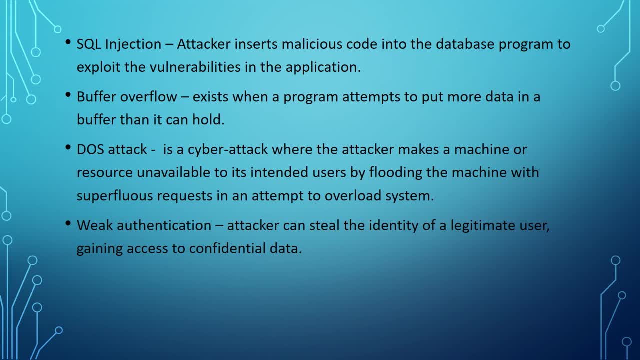 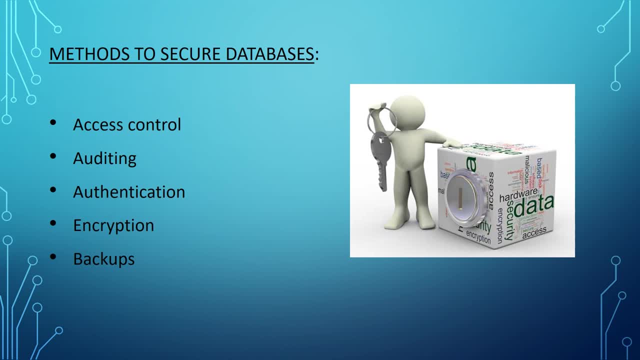 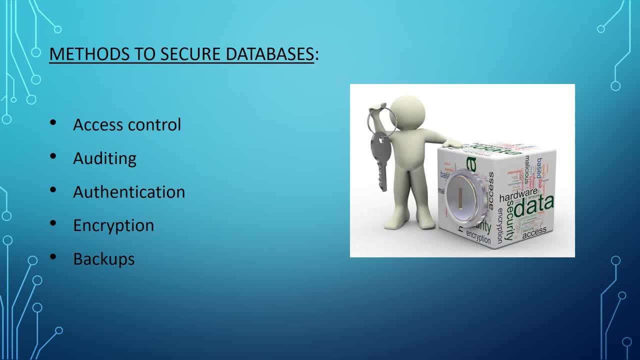 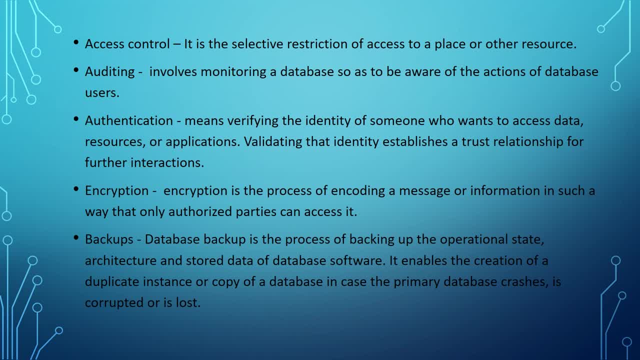 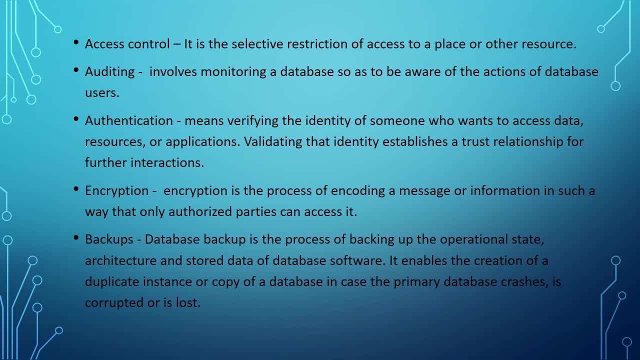 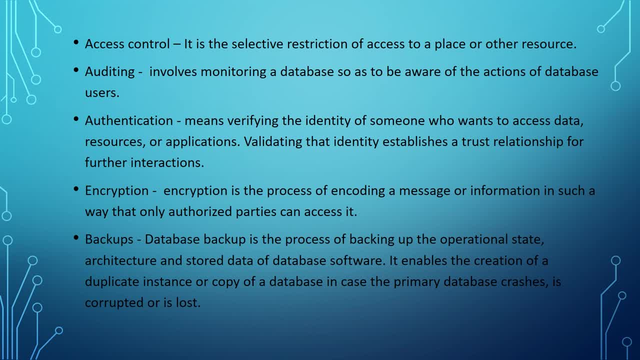 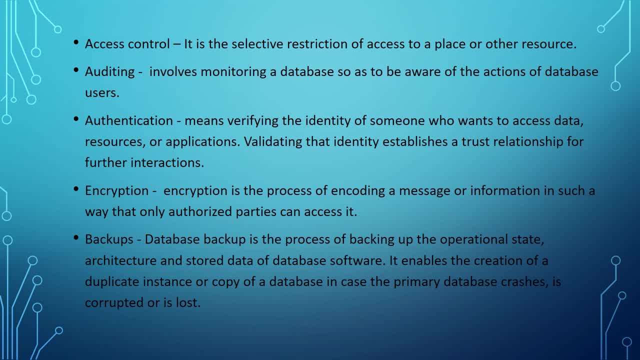 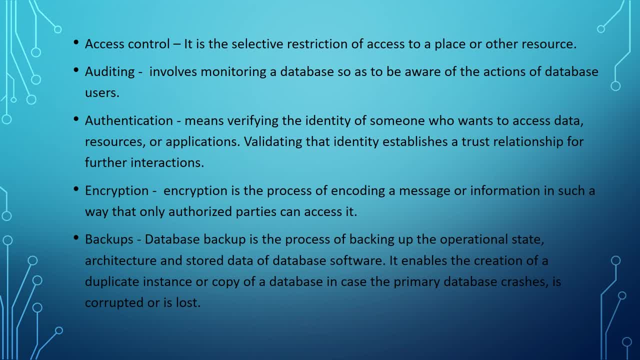 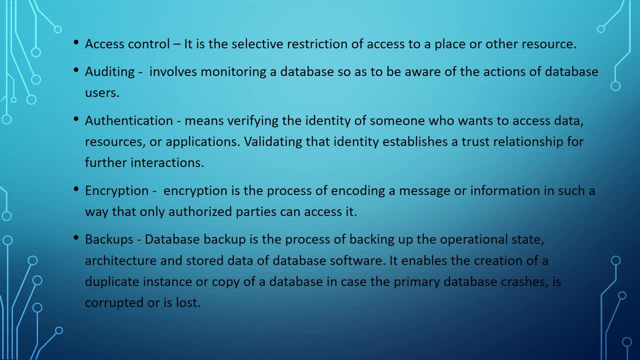 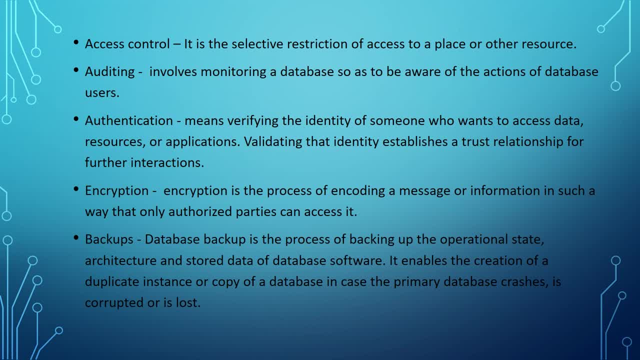 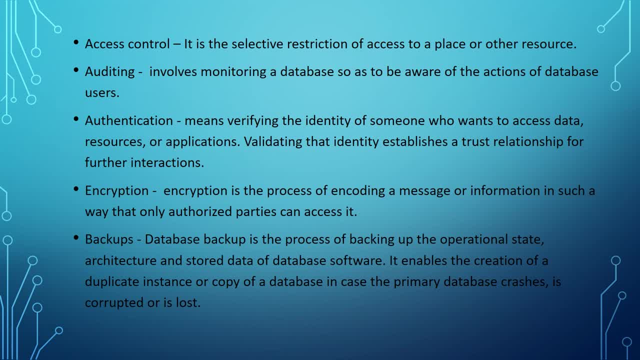 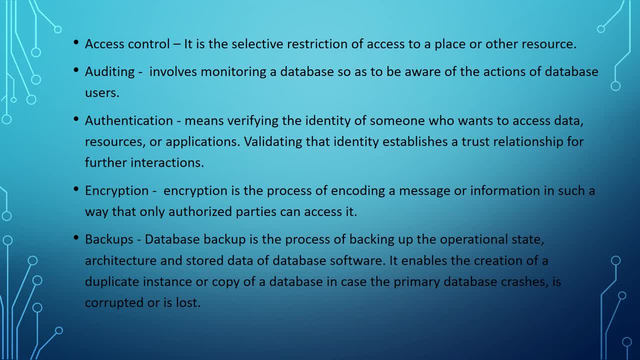 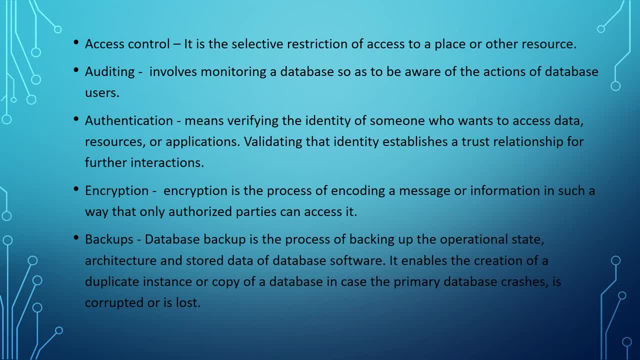 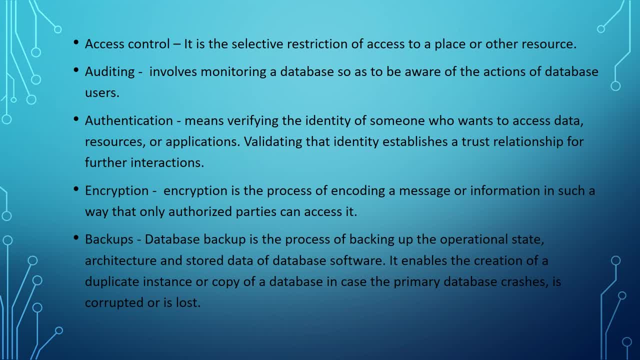 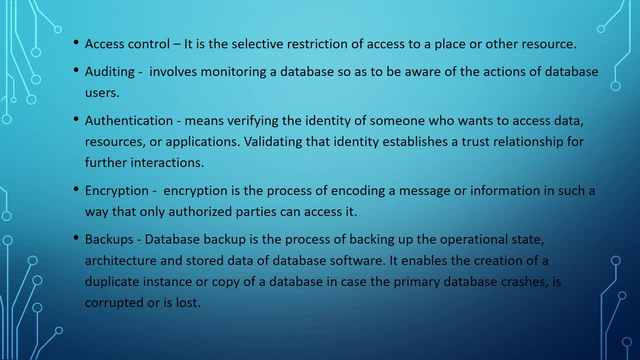 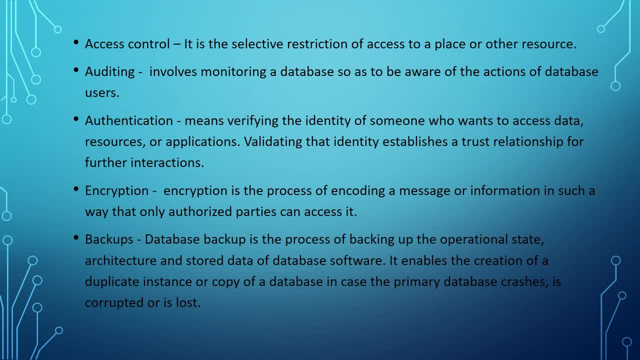 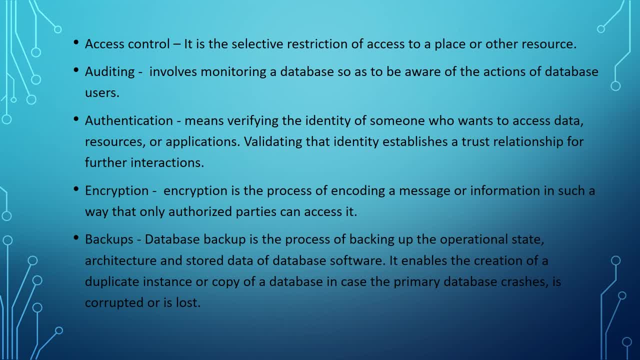 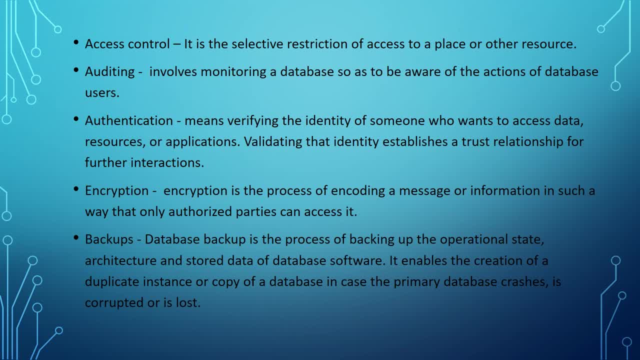 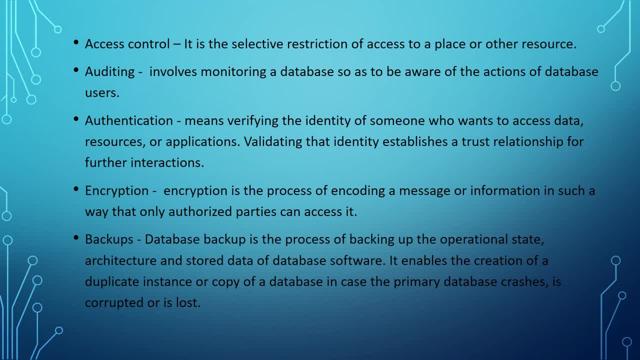 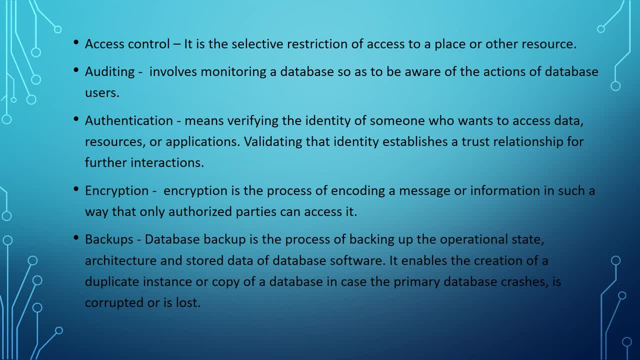 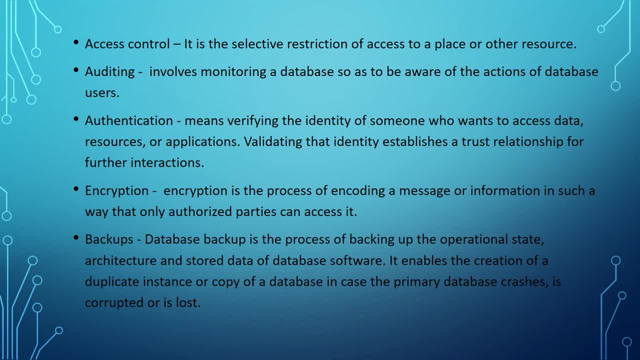 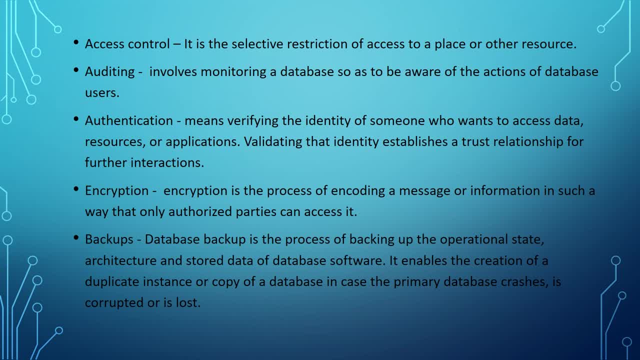 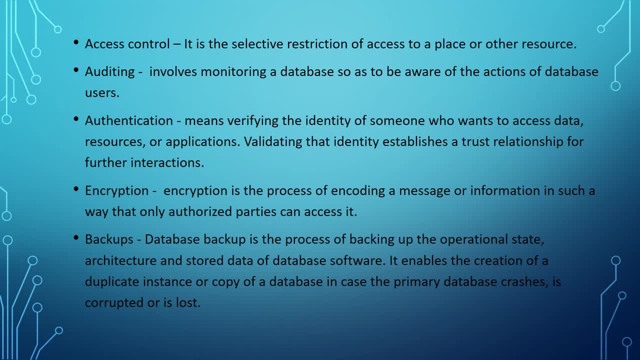 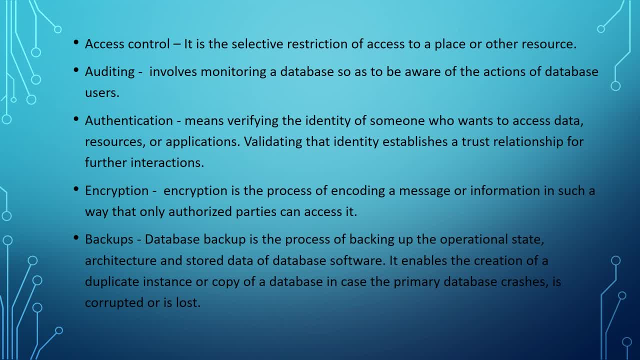 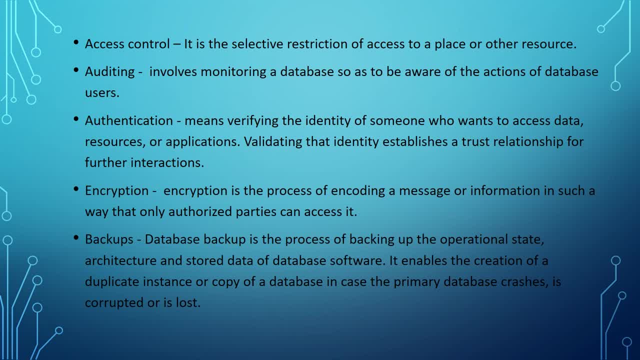 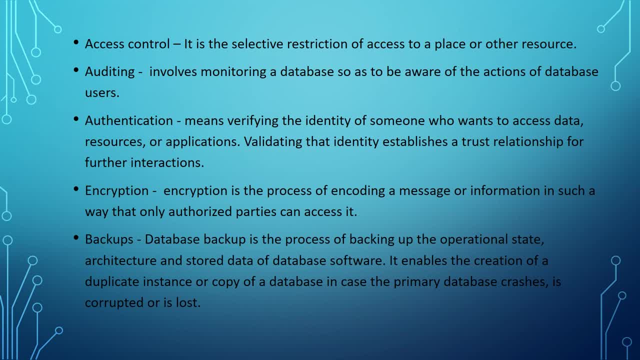 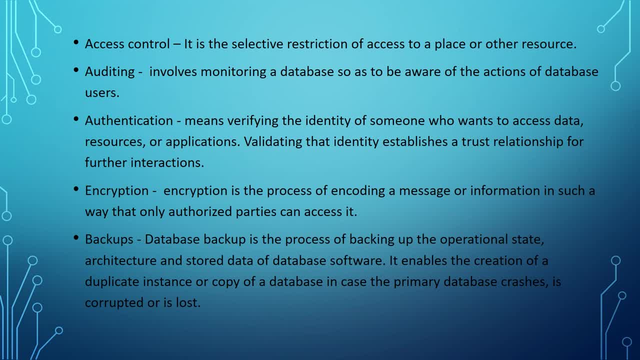 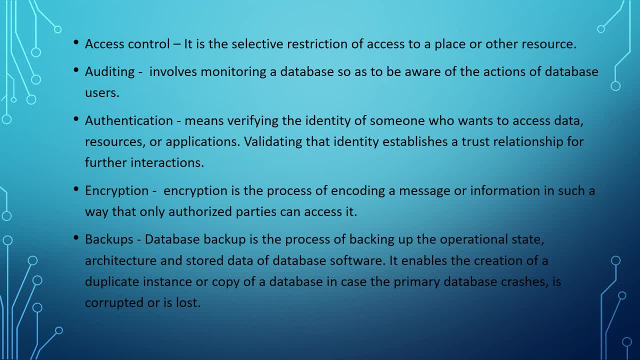 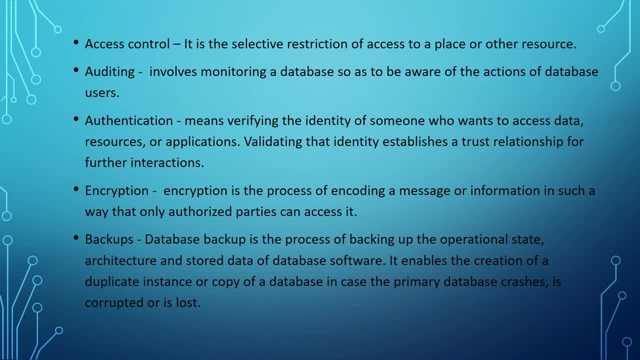 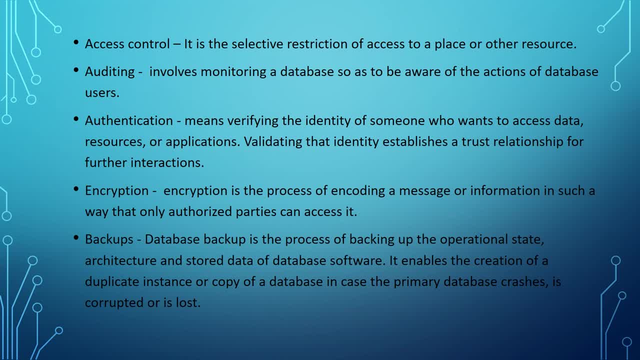